It's kind of a summary of that paper. And the one thing you're going to see, 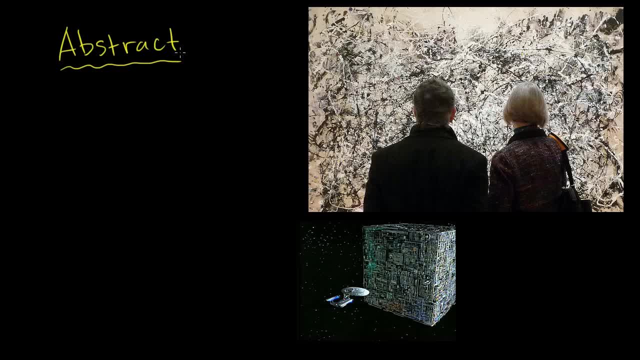 regardless of what context you use the word abstract, there's this kind of notion of taking the essence of a real world object, whether you use it as a noun, an adjective, or a verb. 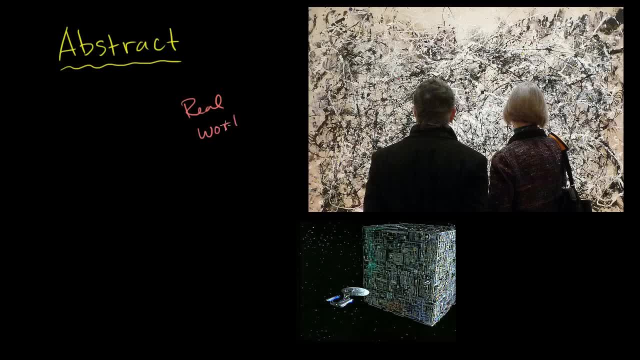 So over here, we have our real world. And then over here, you have your world of you have ideas and concepts. And the general idea behind abstraction, or abstracting something, is you're taking it away from the particular concrete real world, and you're going more in the direction of ideas and concepts. And probably, for me, one of the most tangible ways of thinking about abstraction, which is kind of a contradiction in itself, to think of abstraction in a tangible way, is things. 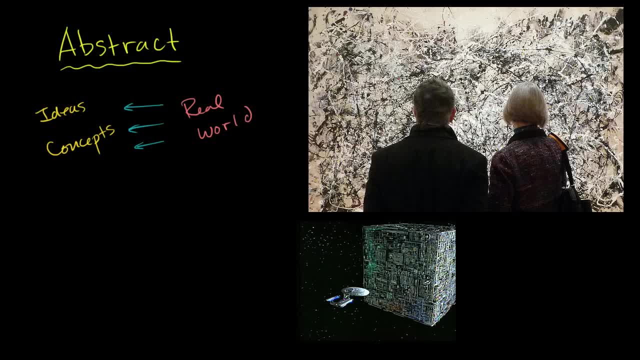 It's things like geometric shapes. So if I were to tell you, find me some cubes, 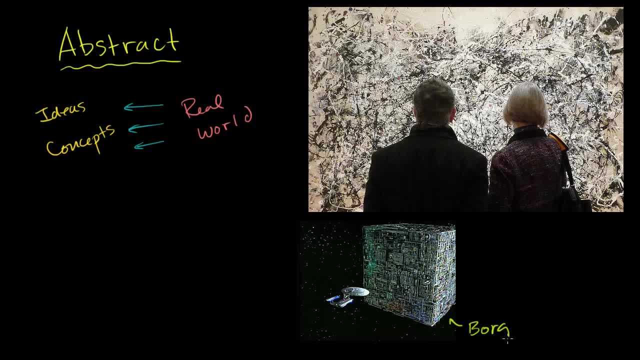 you might point to a Borg vessel right over there. A Borg vessel. 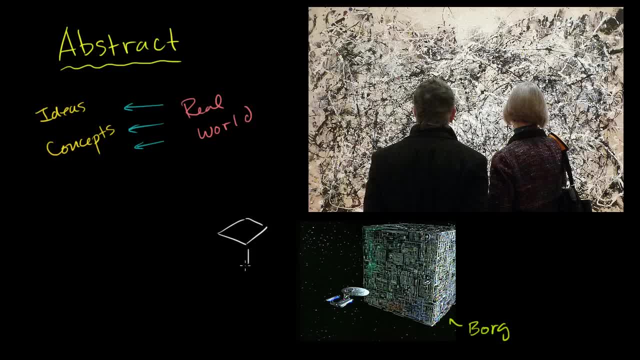 You might point to maybe a pair of dice. 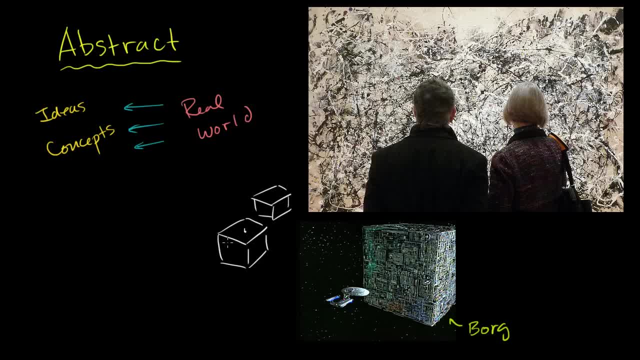 So let me draw the pair of dice. If you are looking for cubes, so you might point to a pair of dice that looks something like that. You might point to a Rubik's cube. 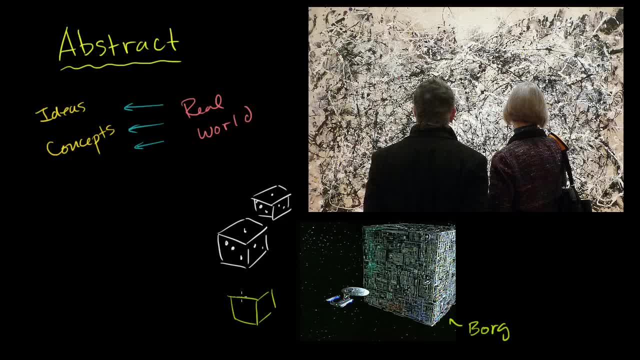 Anything that you could find. There might be a building that looks like a cube. There might be a building that looks like a cube. Or maybe there's a box in your house that is a cube. But in your mind, you have a general idea of what a cube is. You're like, well, I know a cube when I see one. And that general idea is essentially distilling the concept, the idea of what a cube is. All of these things are very different. 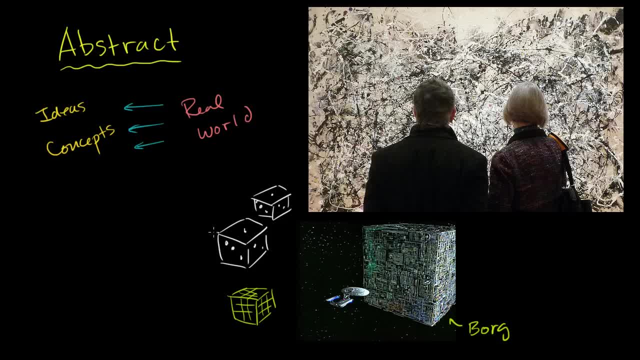 This is some plastic thing that I can hold in my hand. These are these little white things. And they're not even geometrically even close to being perfect. 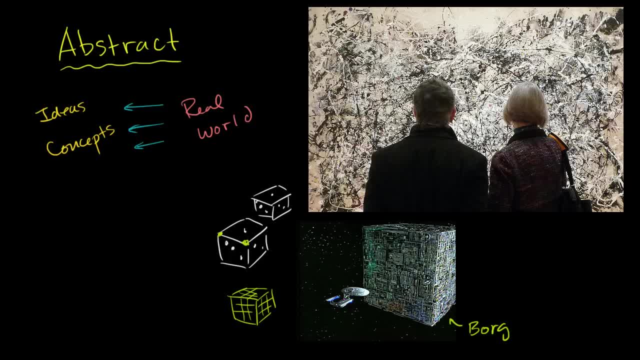 They have these little divots on the side right over there. This is a large Borg vessel. 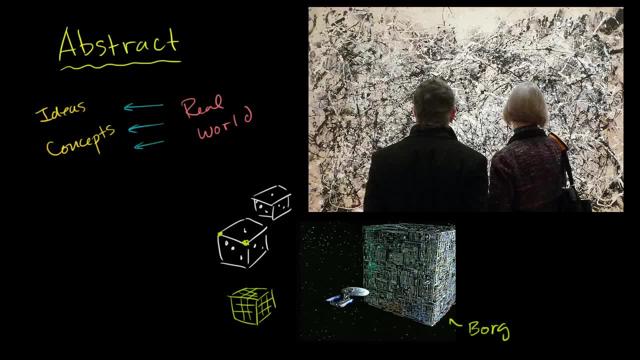 It's not perfect. It doesn't even exist yet. Obviously, it's a fictional thing. 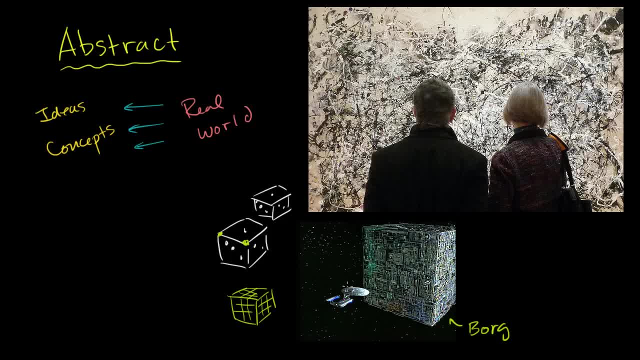 But they all have this cubeness to them. And this is one of the fun things of geometry, is to really distill the essence of these real world shapes. And we do have a definition in geometry, which is an object like this, where every side has the exact same length. So if this is length 1, then that would be length 1. That is length 1. But it doesn't have to be. 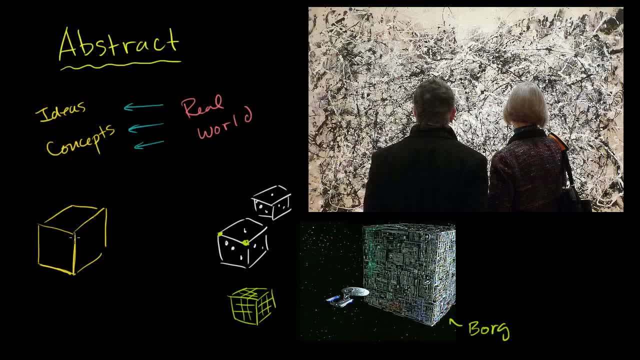 Whatever the length this side is, if it is in this dimension, then in this dimension it's going to be that length. And in that dimension, it's going to be in that length. 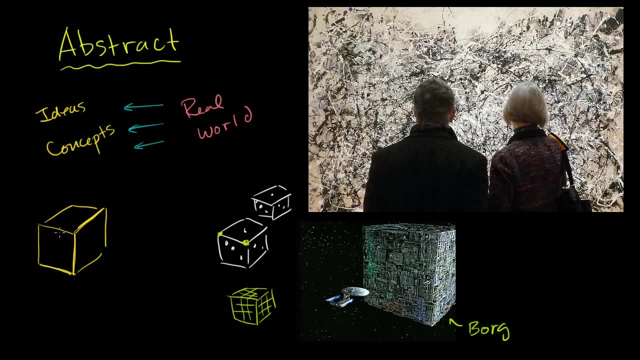 And I'm not giving you the rigorous geometric definition. But I'm just trying to highlight that there is a pure idea of what a cube is. 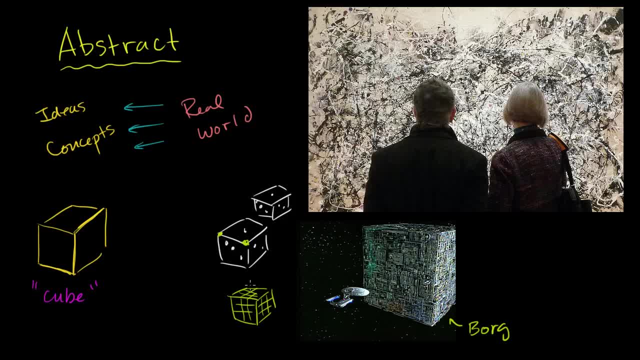 And in the real world, there is nothing that is actually a perfect cube. 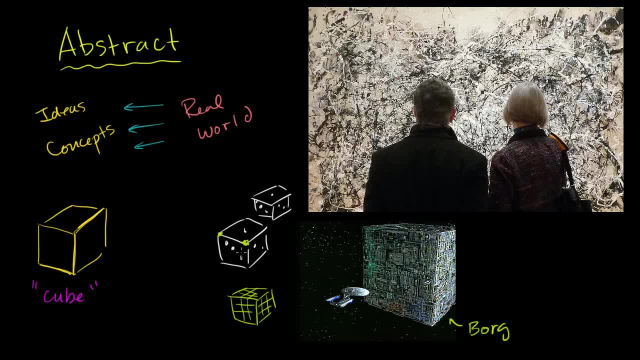 If you were to get really, really close to these dyes, if you were to really try to measure exactly their measurements, they won't be exactly the same measurement. 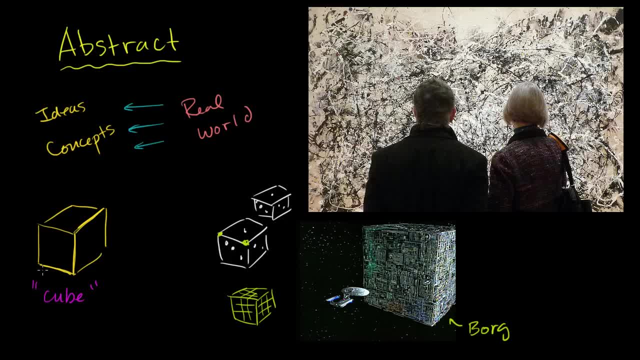 But in the abstract idea of a cube, this is completely the same length as this and this. And actually, this and all of the edges are going to have the exact same length. So this is going from the concrete, the specific, from the real world, if you consider the 24th or 25th century the real world, to going to the idea behind it, the general idea. 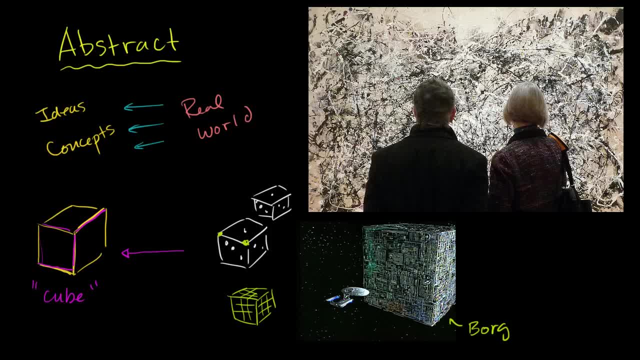 And you've probably also heard the word abstract in terms of art, like abstract art. 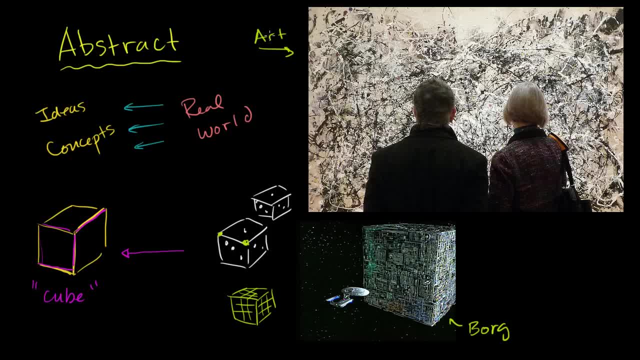 So this is abstract art. And it's the same general idea. If you look it up. If you look in the dictionary, you're going to find 20 definitions of the word abstract. 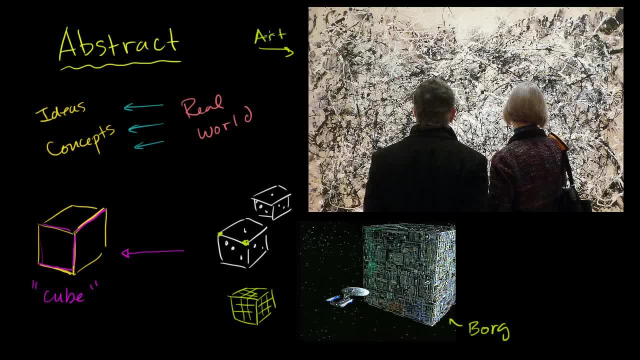 But it's all essentially trying to say the same thing. Abstract art is art that is not focused on trying to paint reality the exact way that reality exists. 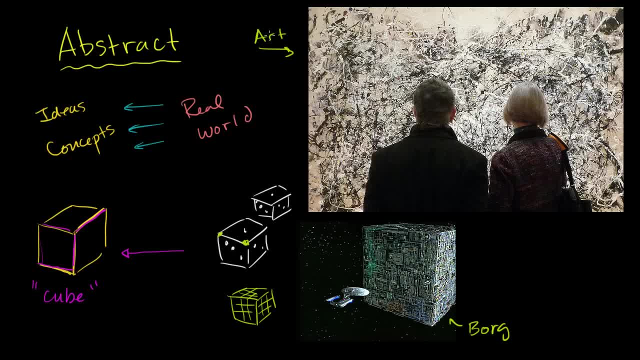 If you look at a lot of Renaissance art, they're skilled at painting figures exactly how they look in the real world. 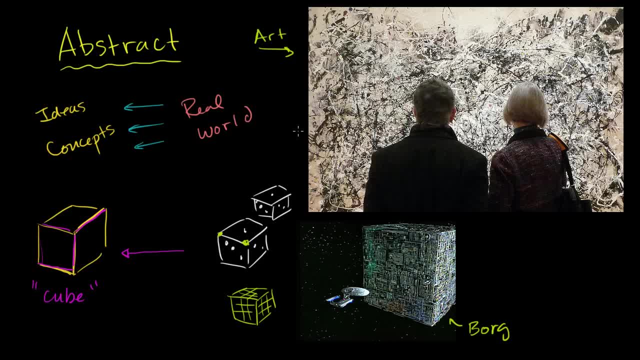 But the abstract artists, sometimes they're not even trying to even represent anything that's in the real world. 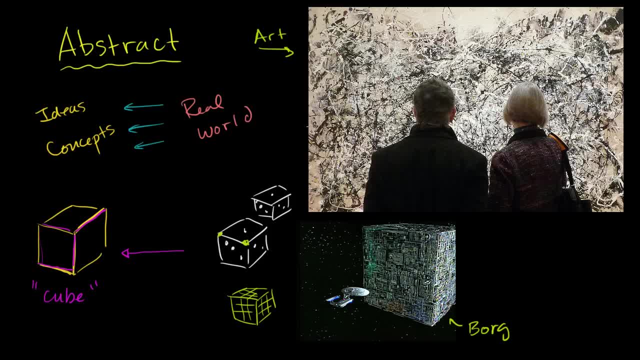 They're trying to represent a raw idea. Or they're trying to represent a raw, raw expression of color, and form, and texture. And this is a Jackson Pollock painting right over here. And I pronounced many, many things wrong. 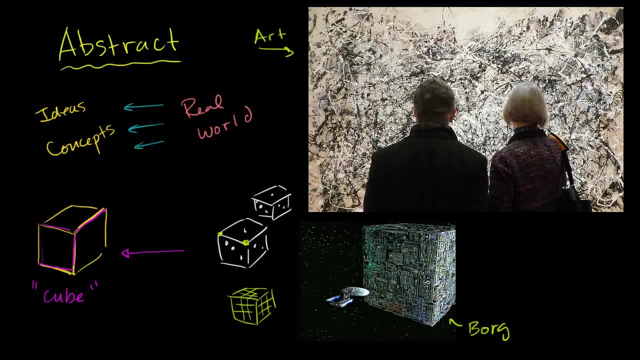 This was taken by our own Steven Zucker, art historian. 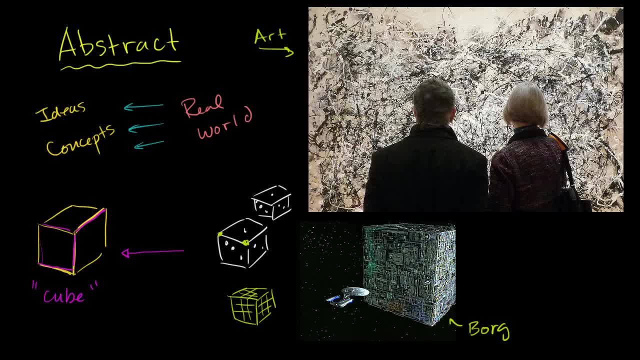 And as you can see, it's not clear. Jackson Pollock is not trying to paint a dog, or a horse, or anything like that. He is painting something that is devoid. It's completely independent of anything that we actually see in physical reality. And the word abstraction, you know, I'm, you know, it doesn't 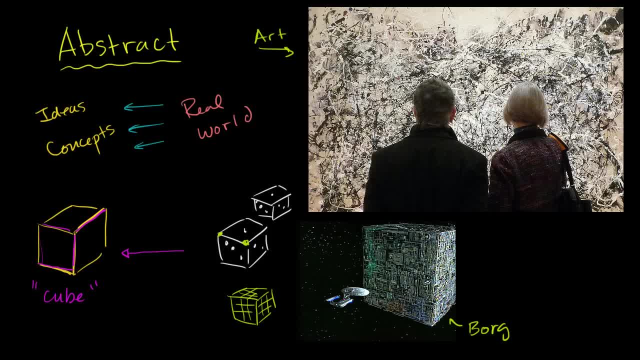 just apply to, you know, pure geometry and art. It applies to almost everything that we do on a daily basis. When we even talk about things, when we even use words, or use symbols, we're essentially abstracting a way. We're abstracting the essence of, of something that actually exists in physical reality. So if I use the word, if I use the word dog, it's a set of symbols. 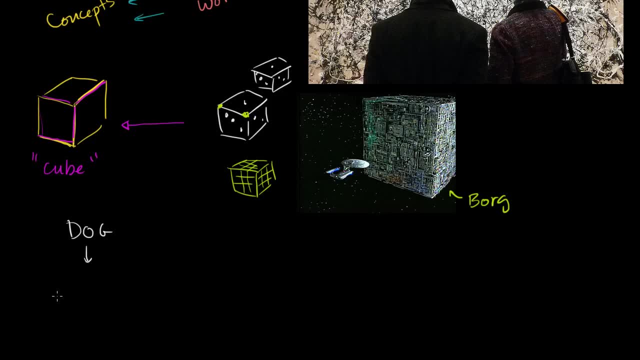 This set of symbols represents something in our minds that we associate with dog. We have in our minds kind of the qualities of what a dog, actually, is. You know, it has four legs, and floppy ears, and you enjoy petting it. And they're man's, or I guess people's, best friend. You imagine this thing called a dog. And it has the essence of dogness, even though when you actually look at dogs in the real world, they look very, very, very different types of animals. 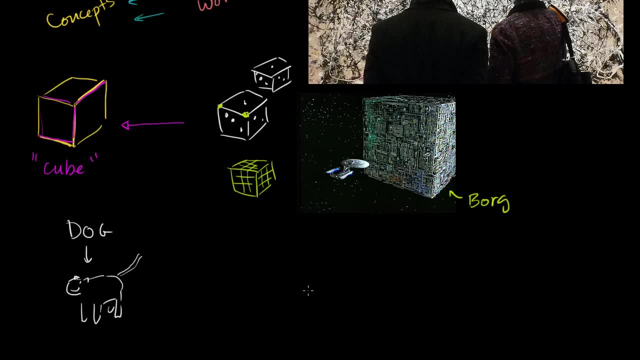 Whether you're looking at a Great Dane, or a kind of a super small poodle. 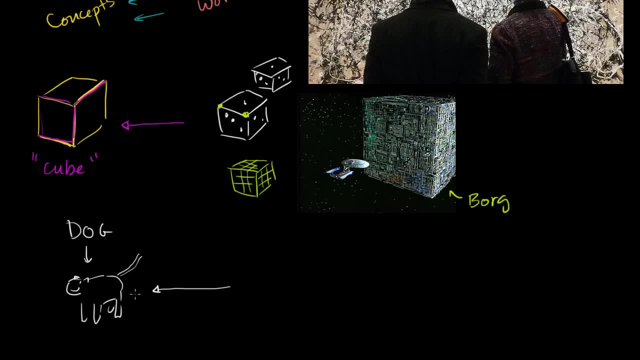 But we recognize there's an essence of those particulars that we can abstract away and say, this is a dog. 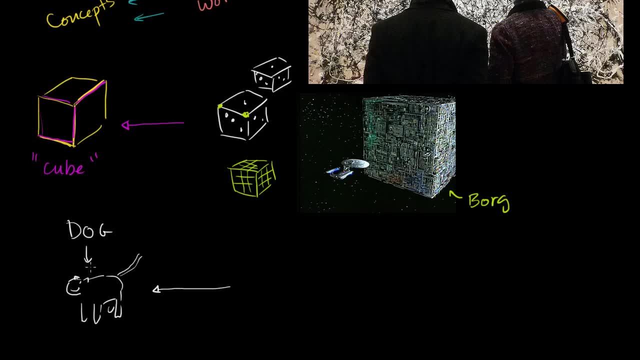 And then we abstract it even more by representing these letter symbols that tend to conjure up this image. 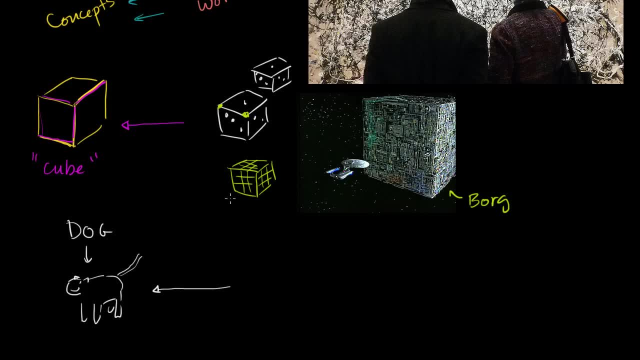 Even when we write something as simple as a number. So if I write the number five, we use it so frequently 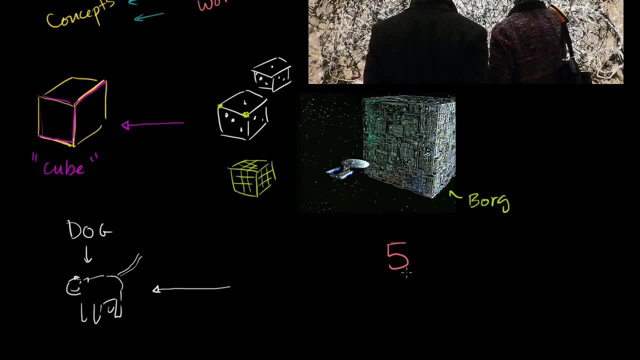 that we just, to us, a number five seems kind of like a concrete thing. 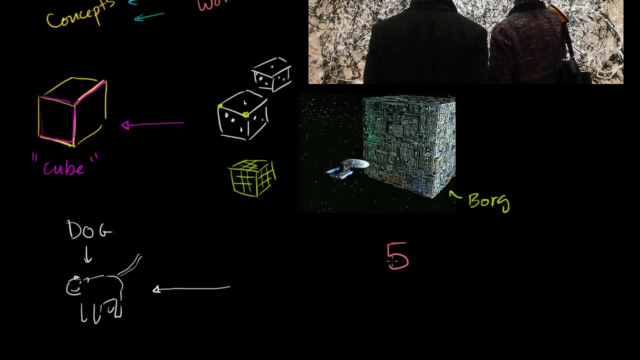 But it's so abstract. It's just a quantity, a quantity of things. I could have symbolized it like that. I could have symbolized five like that. I could have symbolized five in Roman numerals like that. I can symbolize it like that. And in all of these cases, we can say it's the idea of a quantity of five things. 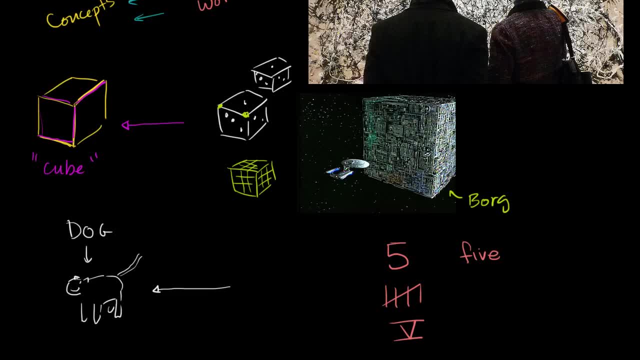 Five, if we were, you could say, point me to a five. 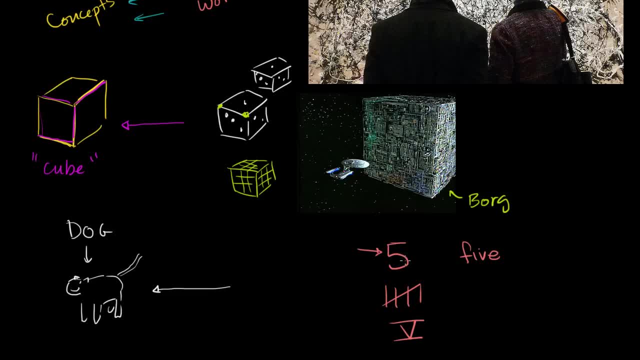 Someone would probably point you to something like that. But they're still pointing you to the symbol of five. But it's still a very, very abstract idea. So hopefully this gives you an appreciation for what abstract means. 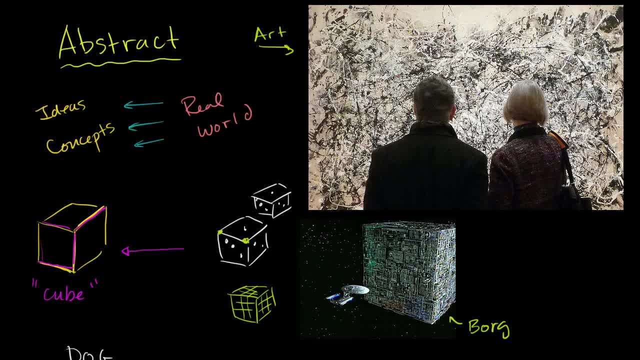 As you can tell, it's kind of a, for lack of a better word, it's kind of an abstract idea. Not to make. Don't be too cute about that. 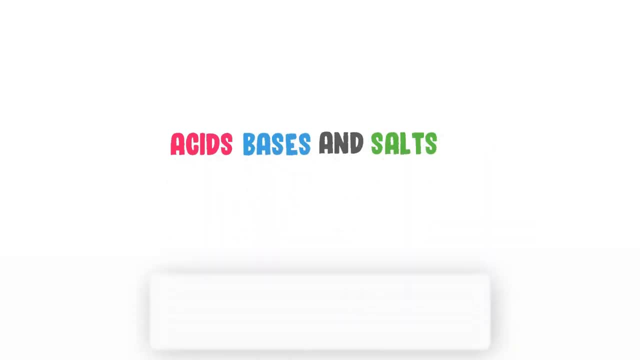 Acids, Bases and Salts Before starting the lecture, click on the subscribe button 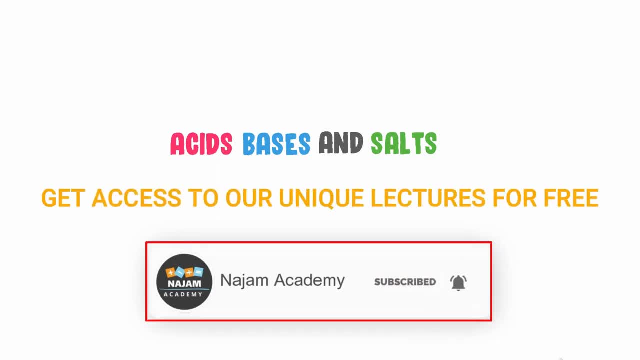 and get access to our hundred of unique and simple lectures for free. 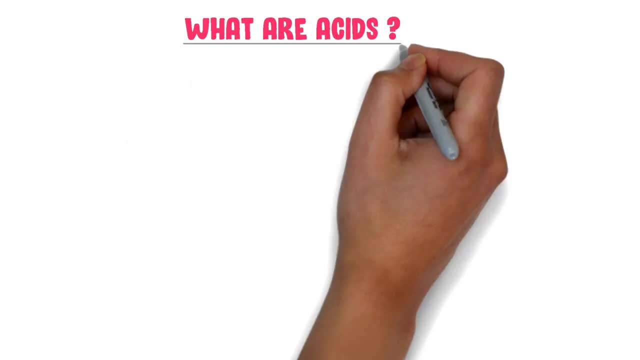 Firstly, let me teach you that what are acids. Well, acids taste sour. They are found in many substances which we use in our daily life. For example, tomato sauce. It contains citric acid. Secondly, milk. It contains lactic acid. It contains citric acid. Fourthly, vinegar. It contains acetic acid. Fifthly, lemon. It also contains citric acid. 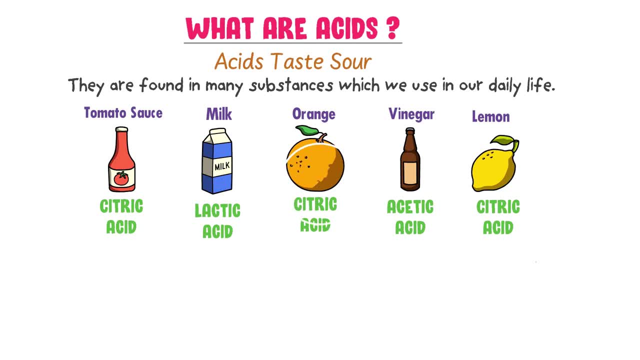 So, different substances contain different types of acids. What about the solubility of acids? 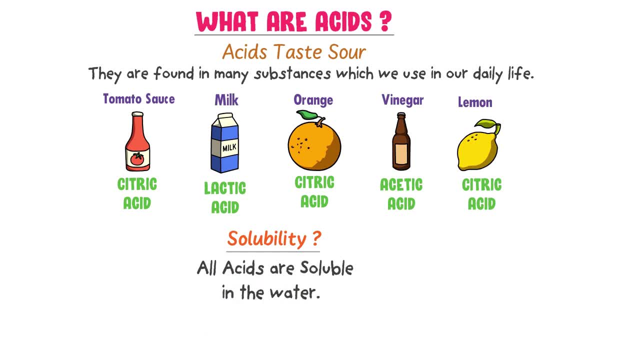 Usually, all acids are soluble in the water. 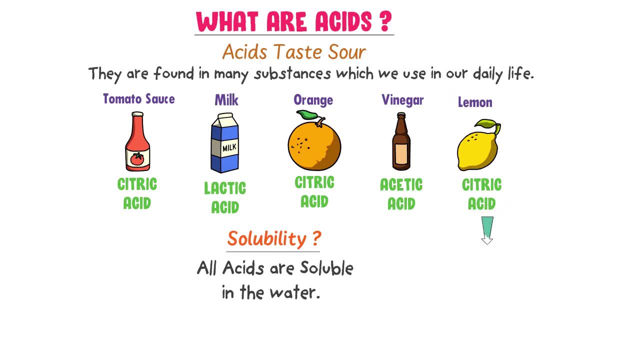 For example, lemon contains citric acid and it is soluble in water. 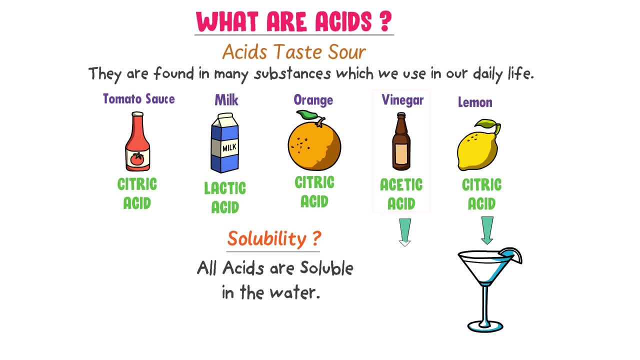 Vinegar contains acetic acid and it is also soluble in water. 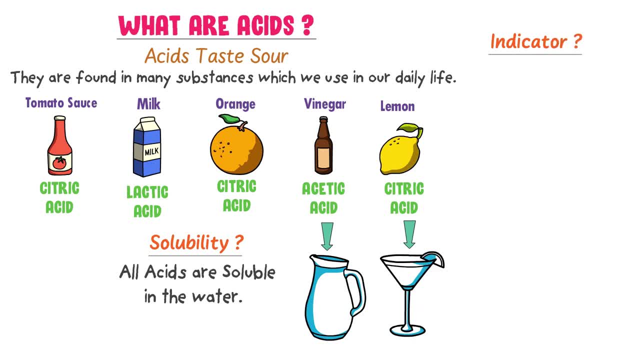 What about the indicator test of acids? Well, there are different indicators used to test the presence of acids, like phenolphthalein and methyl orange. 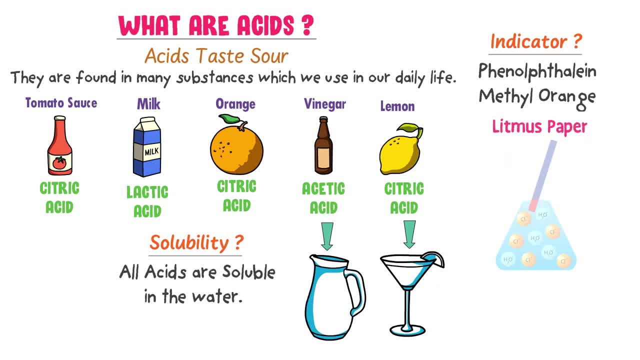 But the most simple and easy test is litmus paper. Acids turn blue, litmus paper red. Let me repeat it. Acids turn blue, litmus paper red. Let me repeat it. Acids turn blue, litmus paper red. Thus, remember that acids test sour. 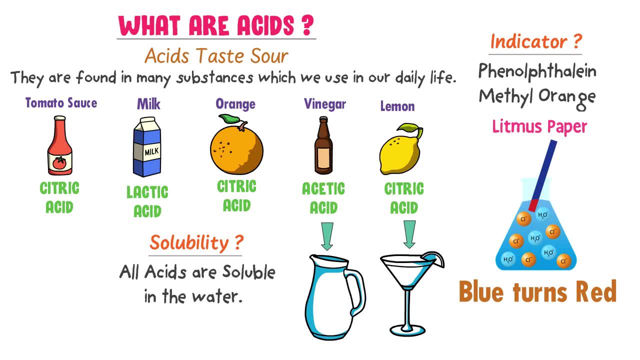 Different substances which we use in our daily life contains different acids. Acids are also soluble in water. And they turn blue, litmus paper red.